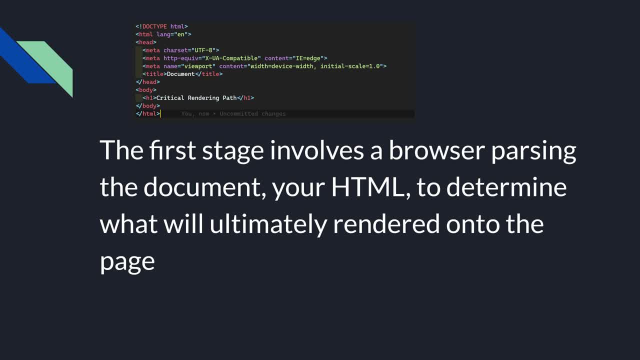 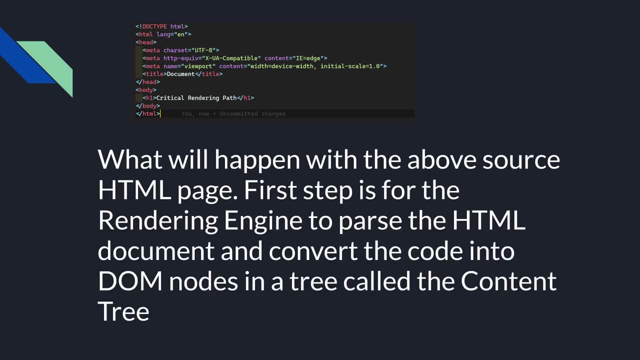 and your html to determine what will ultimately render onto the page. the second stage involves the browser performing the actual render. what will happen with the above source for html page? the first step is for the render engine to parse the html document document, so it will pass the html document and convert the code into your dom. nodes in a tree. 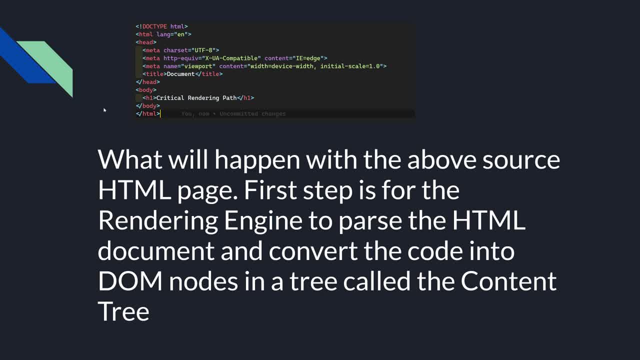 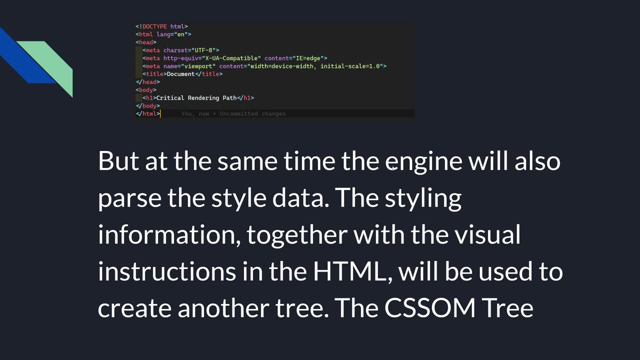 called the content tree here. actually it's a render tree. so here, what is what i am trying to say is the html document what it is there. so the rendering engine will parse the html document and convert the code into your document, dom nodes, but at the same time the engine will also parse 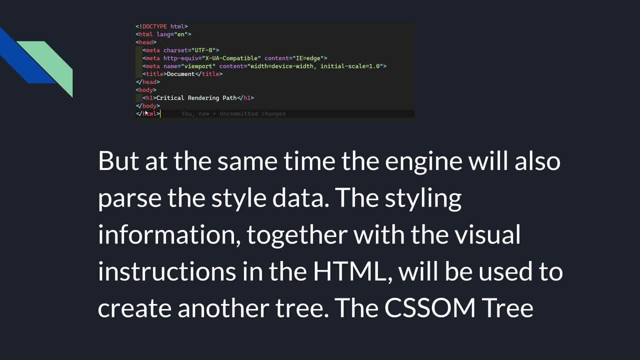 the style data. so when this html document is transferred to the html document, it will山 document is passing the engine also, the rendering engine also parse the style data. that is nothing but css. the styling information, together with the visual instructions in html, will be used to create another tree. that is nothing but the css arm tree. finally, the dom tree and the css tree. 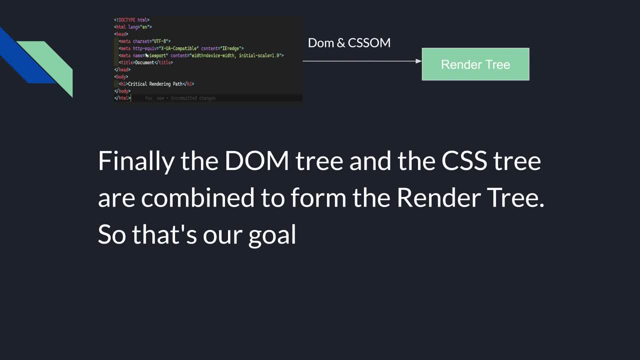 are combined to form the render tree. so here i am trying to say so: first, the html parser will parse the html and convert into dom. simultaneously the style data also will be parsed by the rendering engine to convert it into a css arm. so these two trees can finally forms the render tree, so that 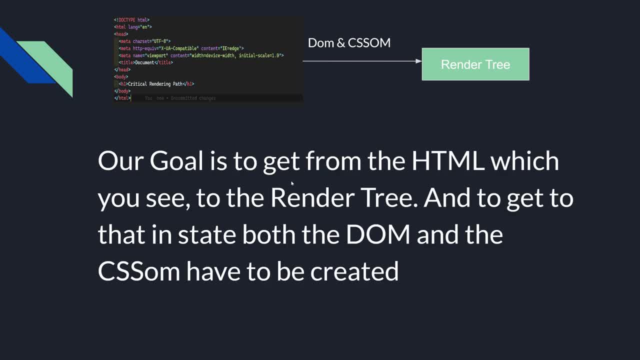 is our goal. our goal is to get from the html which you see, to the render tree. so our goal is: this is the html, and we need to construct the dom and css and we need to generate the render tree and to get to that, instead it- both the dom and the css arm- has to be created. the next goal is actually displaying the data. 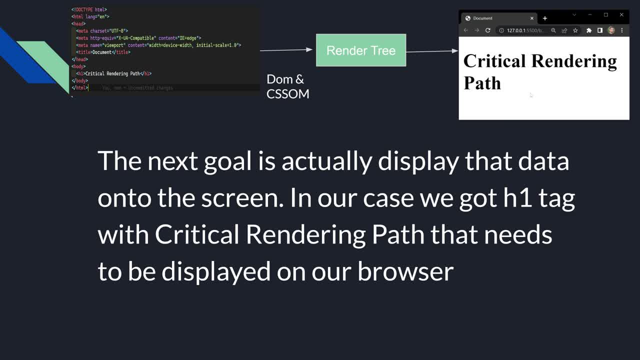 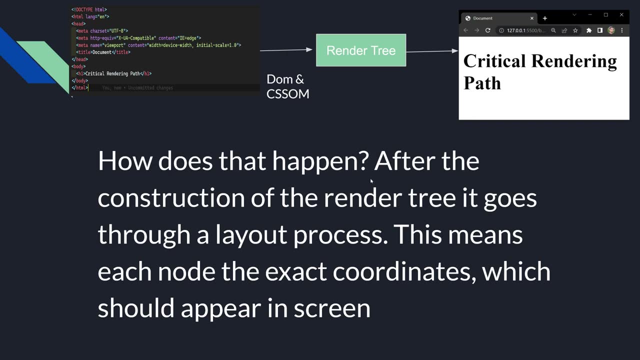 onto the screen. so render tree is created and now we need to display the data onto the screen, in our case, the html. we got the h1 tag which contains the content critical rendering path, and that needs to be displayed on our browser. so that is the thing. how does this happen? 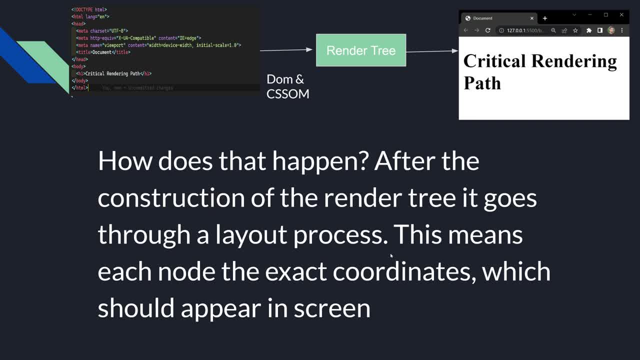 after the construction of the render tree, it goes through a layout process, we know right layout process, and also last one is the painting process. so the next process is the layout process. this means each node. the next, this means each node, the exact coordinates which should appear on the 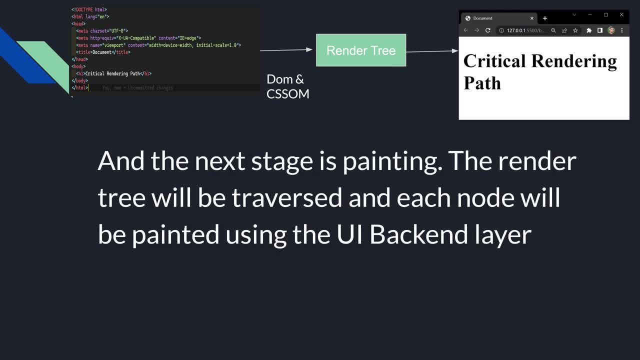 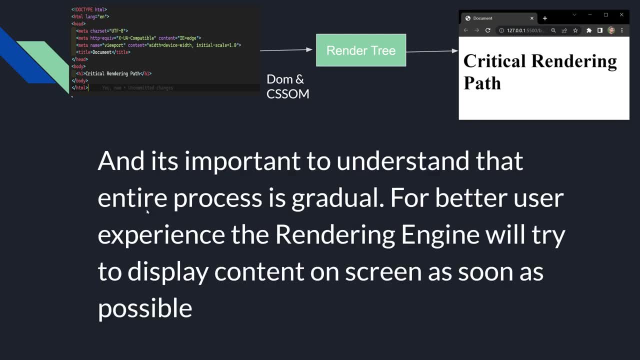 screen and the next stage is the painting. the render tree will be traversed and each node will be painted using the ua backend layer, and it is important to understand that the entire process is gradual. so the entire process, what you are trying to see, is gradual one. 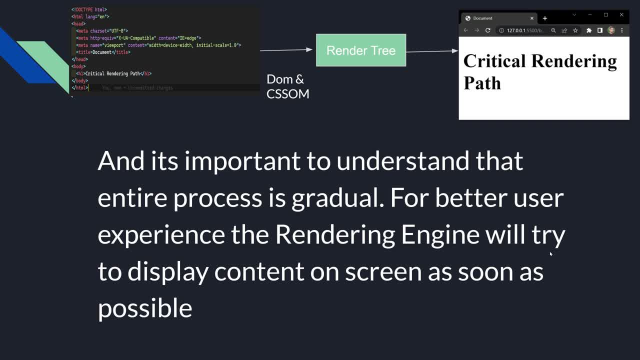 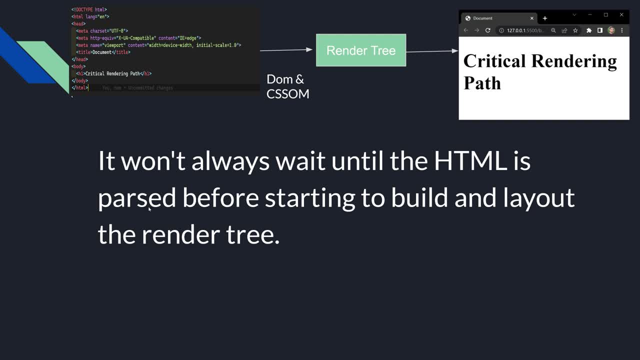 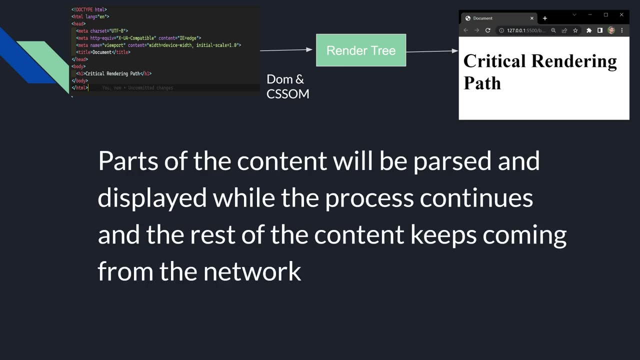 by one. it will do for better user experience. the render engine will try to display content on screen as soon as possible. it won't always wait until the html is passed before starting to build and layout. before starting to build and layout the render tree, parts of the content will be passed. 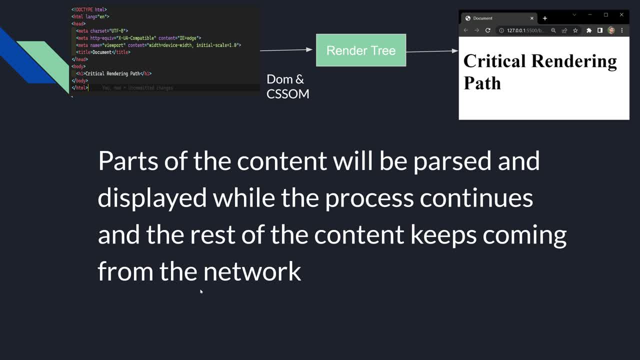 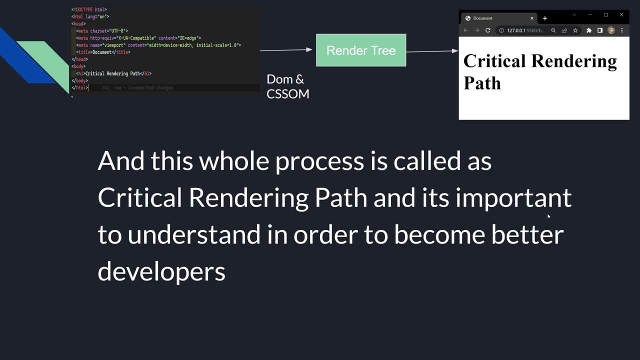 and displayed while the process continues and the rest of the content keeps coming from the network, and this whole process is called as an critical rendering path and it is important to understand in order to become a better developers. so this is all about the critical critical rendering part. so what is this critical rendering path? what i am trying to explain you is: 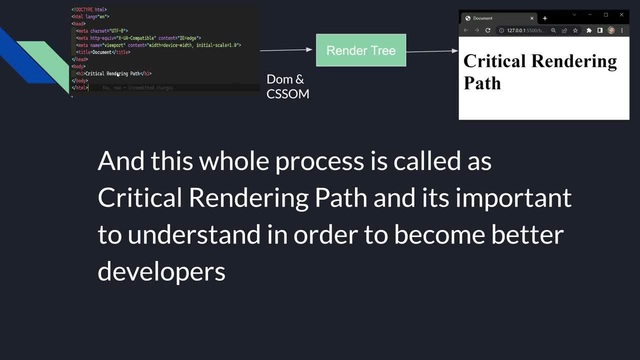 the source html which you are having. so first the rendering engine will parse the html and it will convert it into a dom tree and also by simultaneously, the css data. the style data is also converted into a css arm tree by the rendering engine- only both the tom tree and css tree when. 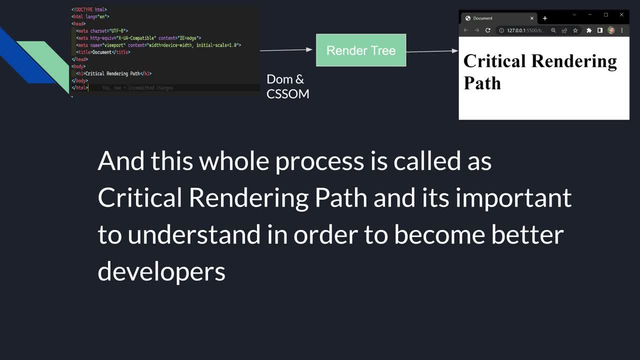 it is created. so then the render tree will be created. so in order to create the render tree, we need to have the dom and css be ready. so after creation of this render tree, now the layout process occurs. the layout process will try to understand so where the each node in the viewport. 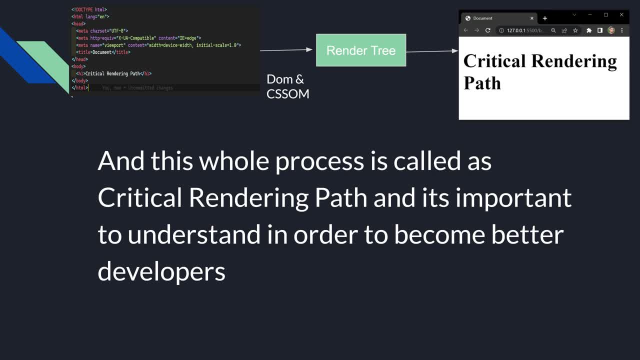 should exactly fit. it will determine the position of those all things. after finishing of the layout process, now the painting process goes on. so now the delay, now the position has been declared by the each node and the things will be going on, painting one by one. this is how. 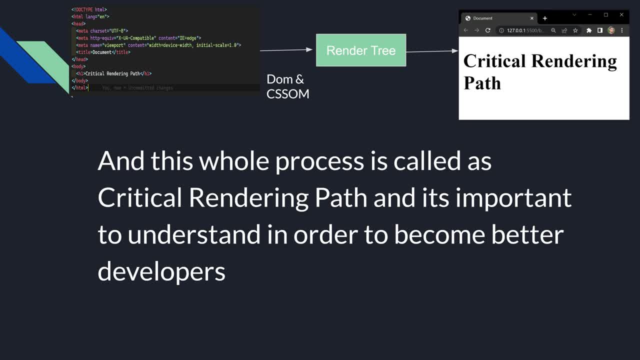 actually the display of the. this is how actually the browser functionality works, and these all the process is gradual, so parts of the content will be passed immediately. the layout will be determined and it will be painted so like this: so it will not wait until the total html is parsed and total css arm. like that it will not true, so the part will come.